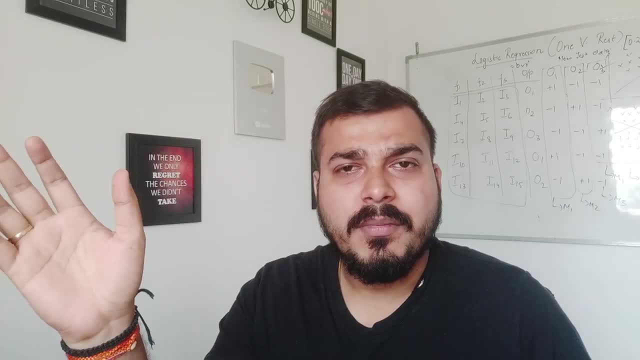 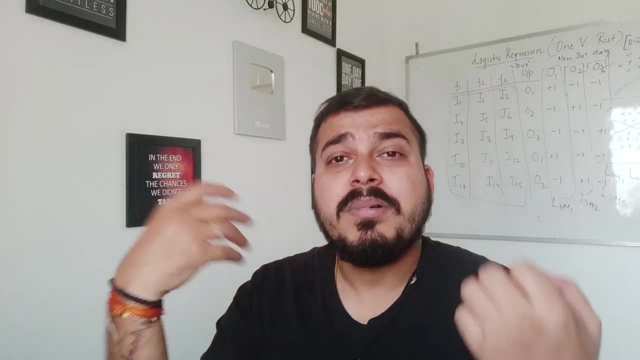 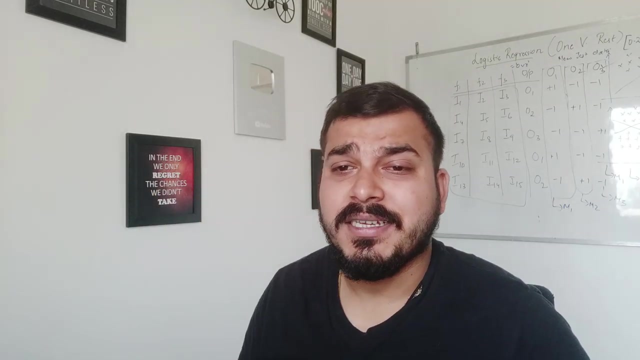 to remember the formula. guys, you do not remember the formula, but understand the formula, the concepts, how it is actually used. you need to explain only those, because it is not- it is not- compulsory to remember the formula, for that Google is already there. but if you know the concepts, it is well and good. now the next thing is that, what? 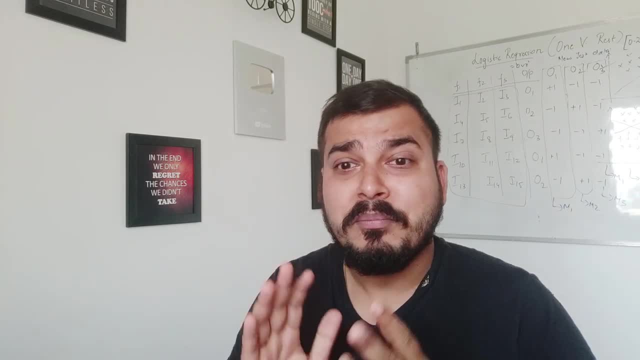 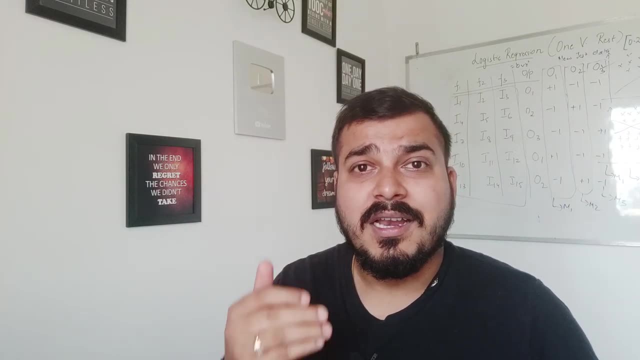 this was the most important thing that was actually asked to me and in many interview questions. suppose in in your data set you have features f1, f2, f3, f4 and some of the features are numerical values and some of the features are category values. how does the decision tree is getting constructed for? 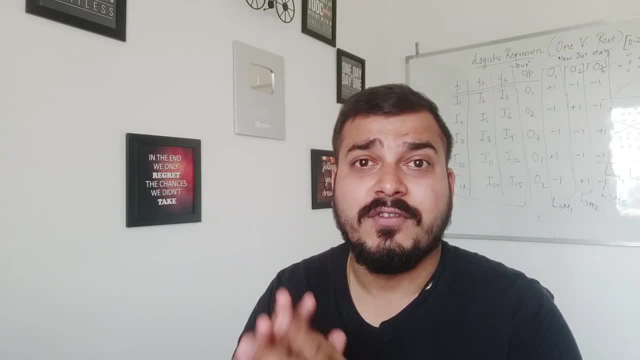 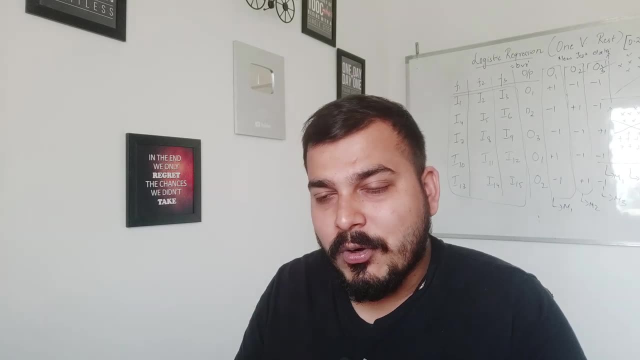 category variables, how a decision tree is actually constructed for numerical variables. and again, guys, I have uploaded all this particular video in my youtube channel. the reason why upload I upload those videos is that because those were the questions that were asked me in the interview questions. right? so that is the. 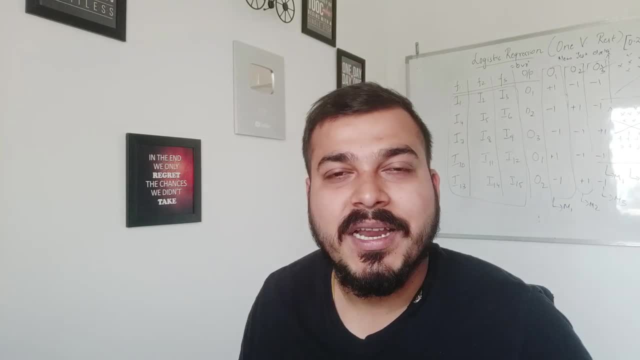 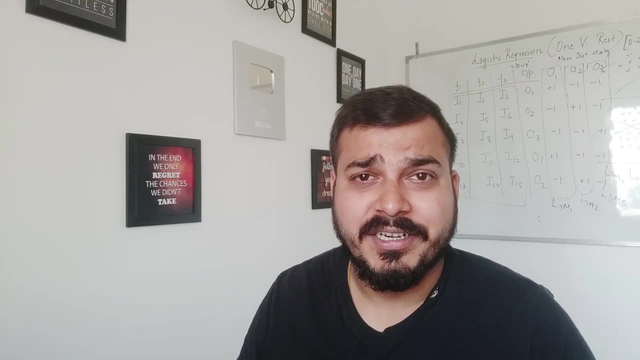 main thing- that is the main purpose of my channel- is that you should be able to get the job quickest possible. so you need to understand- you need to explain them- how category features are actually splitted, on how decision trees are constructed and, based on numerical features, how the decision trees are. 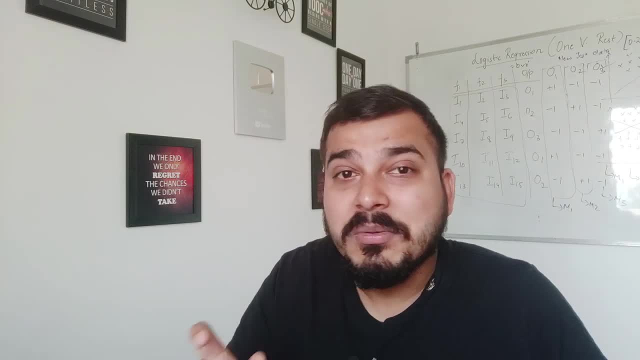 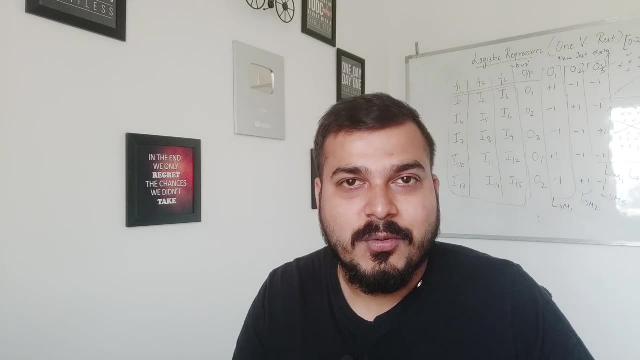 actually constructed. this is a very, very important question. that about the numerical features: okay, because I see many people know about category features. they directly explain the concept. okay, by using entropy or Gini, impurity or an information. again I can construct. but in case of numerical features you need to. 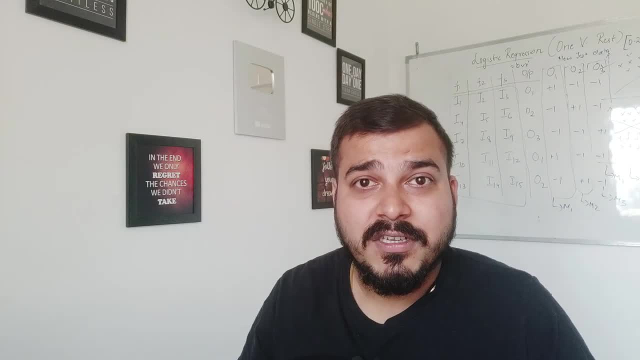 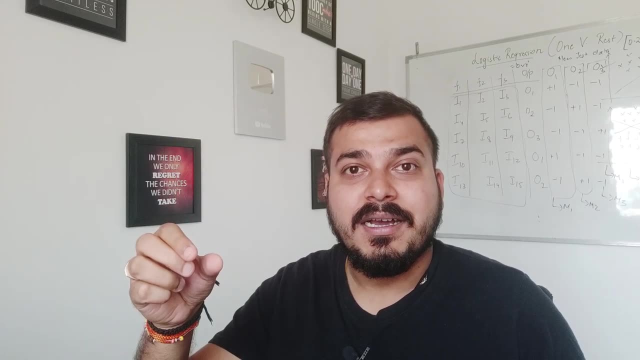 consider each and every example. so suppose if I, if I have many numerical features, I'll go from the top. I'll take the first one, put it in my left node, remaining all values put it in my right node, then I'll go to the second uh record. I'll put that and the top record in my left node and then my right node. 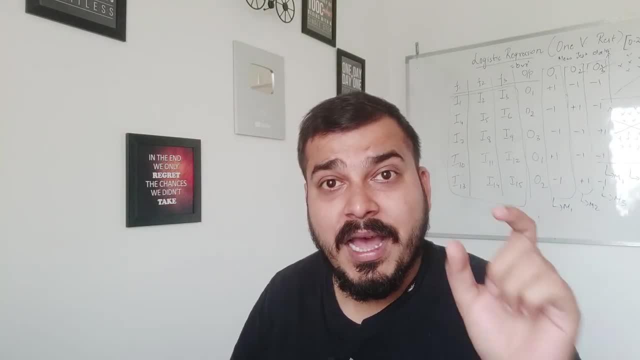 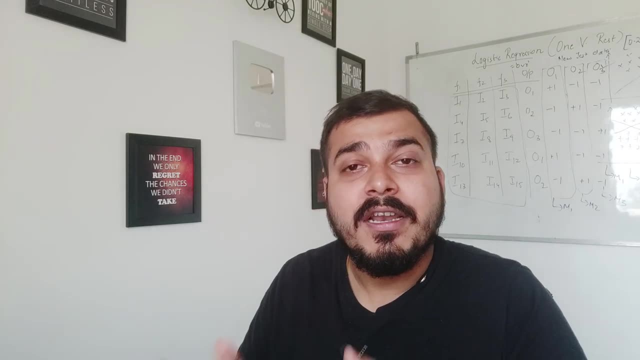 and considering all these particular scenarios, I have to split. I have to split with each and every records. considering all this particular scenario, I have to go and find out the information gain and which is actually giving the very, very good information gain value. I have to take that okay and 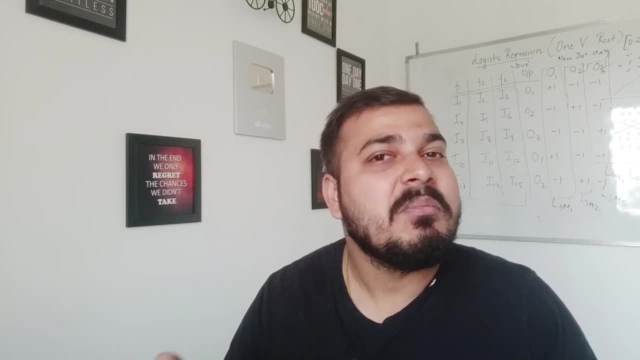 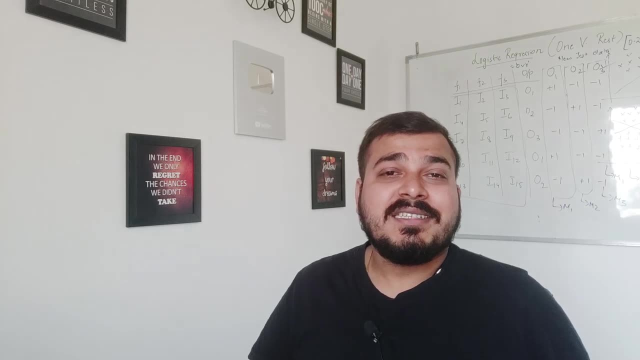 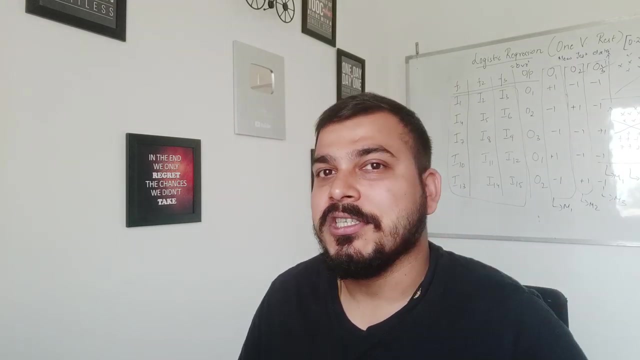 still, if you have not understood it, go and watch my video in my complete machine learning playlist about decision trees, I have uploaded three videos on that. you'll be able to understand it now. the next thing is that- and this is this is also very good questions- okay, what is the impact of outliers on decision? 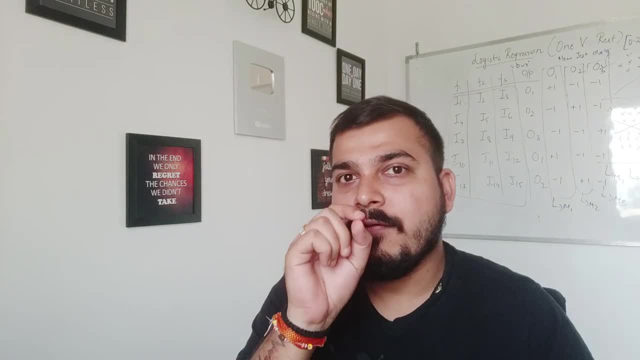 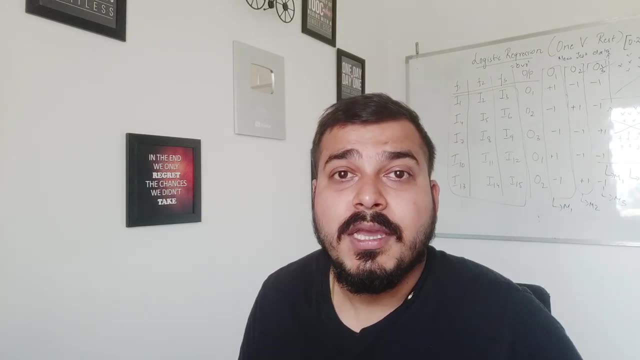 trees. I would like to ask this particular question to you all, if pleased to comment down in this particular video. if you know the answer, I'll have a look and I'll again give you back a reply for that, okay. so what is the impact of outliers for indecision trees and how do you actually remove the impact of in? 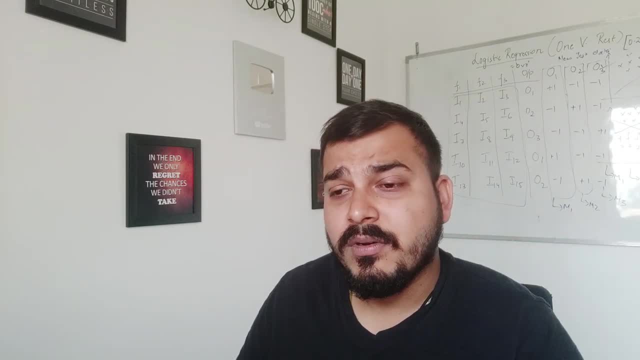 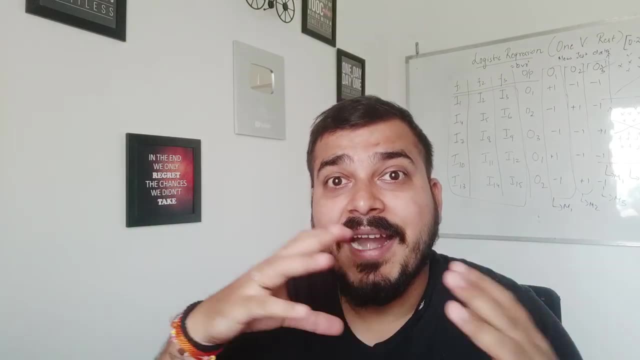 outliers. so these are the two questions that I would like to ask, please, to comment down in this particular video. the next thing is that some of the properties of decision tree- you should know that decision tree usually have low bias and high variance. now, what does this exactly mean? because they'll ask: 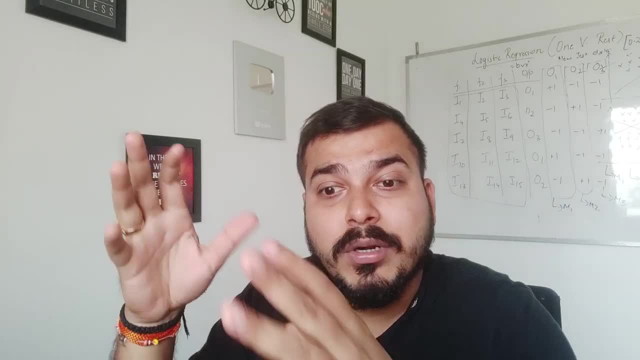 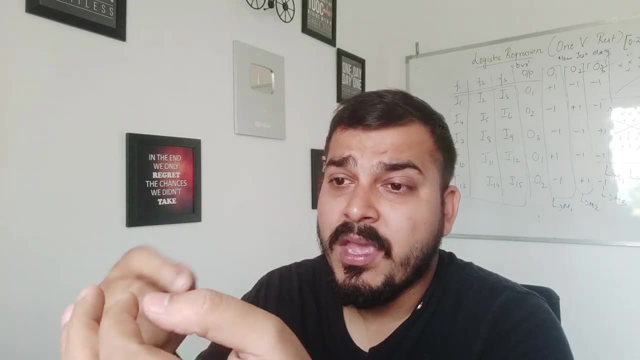 you this question and you have to tell them how you are going to reduce this, how you are going to make this high variance to low variance. okay, this is pretty much important, also to make them explain now what is low bias and high variance. you heard of underfitting and overfitting, like 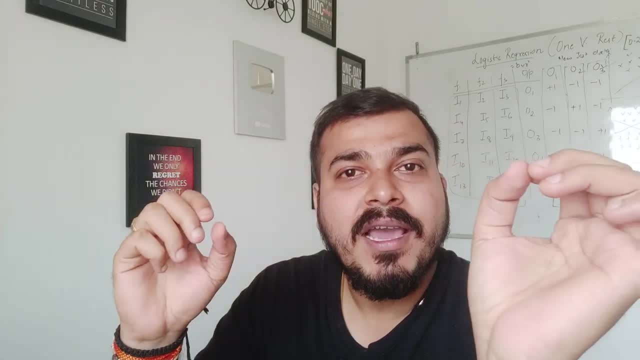 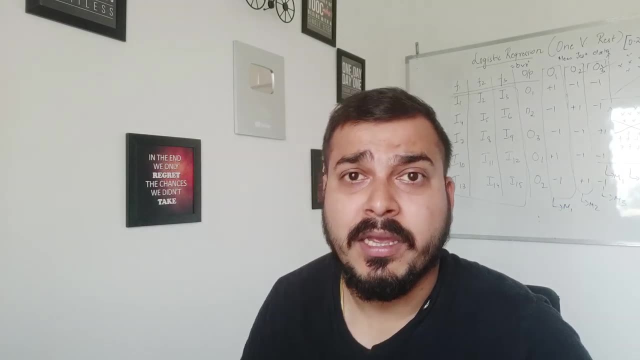 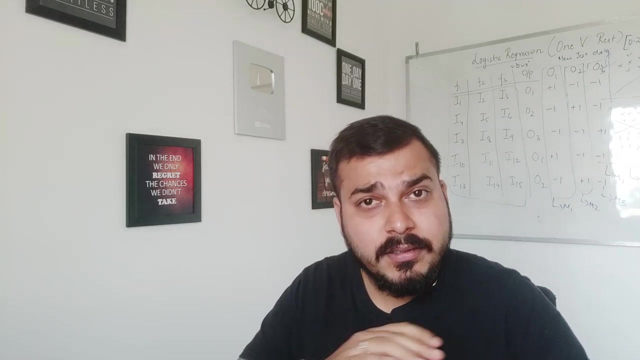 and a generalized model should have exactly low bias and low variance. but decision tree exactly gives us low bias and high variance if you are not applying any hyper parameter tuning. that basically means if you are dividing the decision tree with, with the respect, with respect to the number of features that i have, till the depth, till all the depth, till the leaf node, in short, okay. 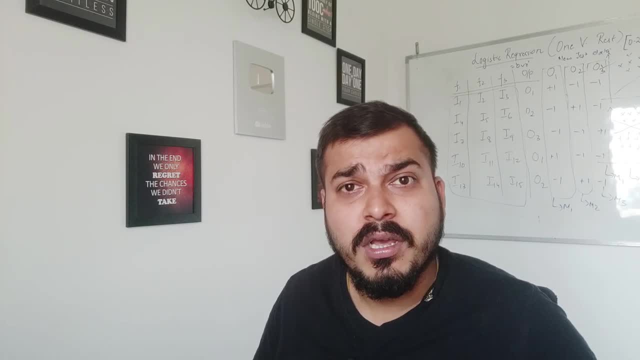 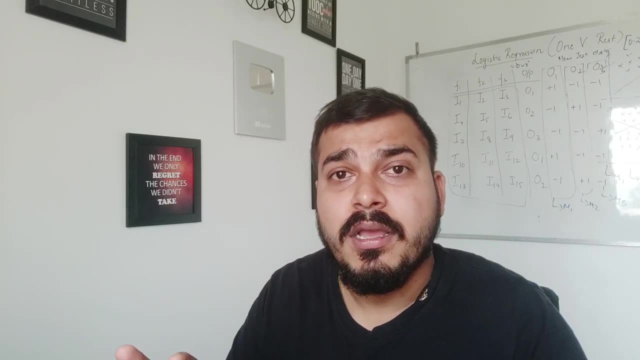 if i divide those features based on till the leaf node, okay, that basically means that i'm getting high variance. that that in short says that i'm training my model for the training data in such a way that will give us good accuracy result for training data. but whenever my new 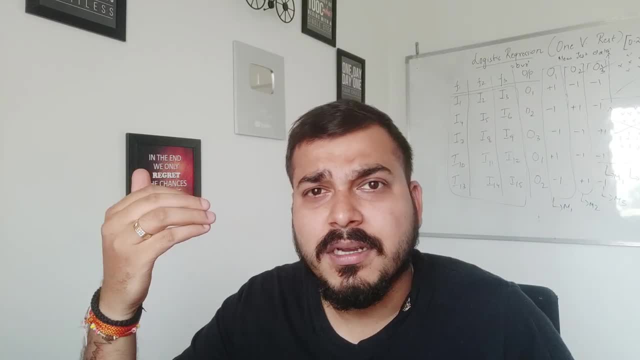 technology is used, i'm getting high variance. so that basically means that i'm getting high variance. so that basically means that i'm getting high variance so that when the test data comes, you know at that time it will not perform well, it will give us a little bad accuracy when compared. 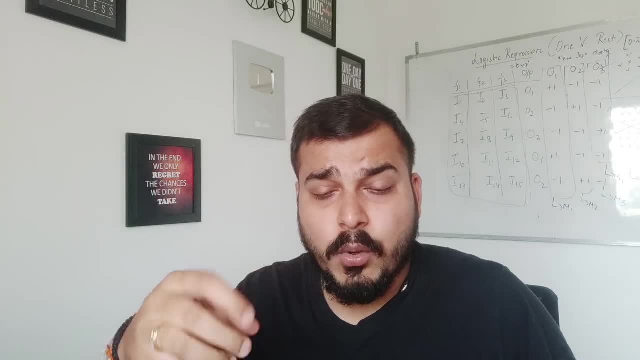 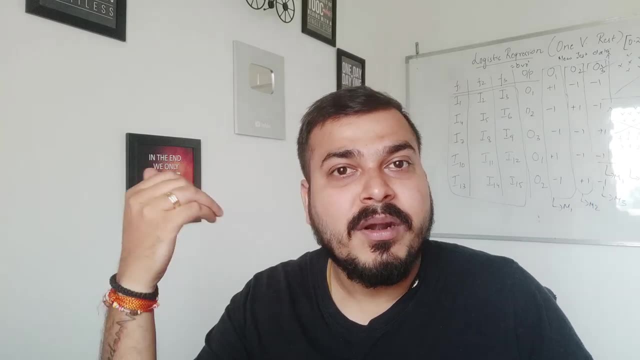 to the training data. so this is just a case of overfitting where your training data has got trained very, very much properly. my model has learned the training data in much of a better way, but for the test data it was not able to predict, so you need to explain them. what is this low bias? 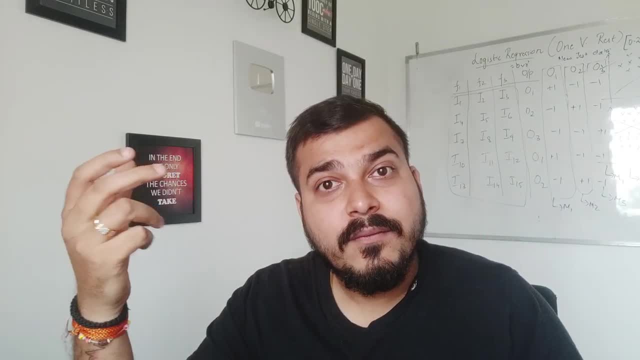 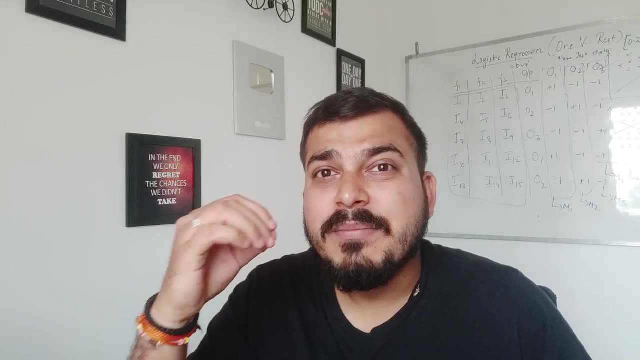 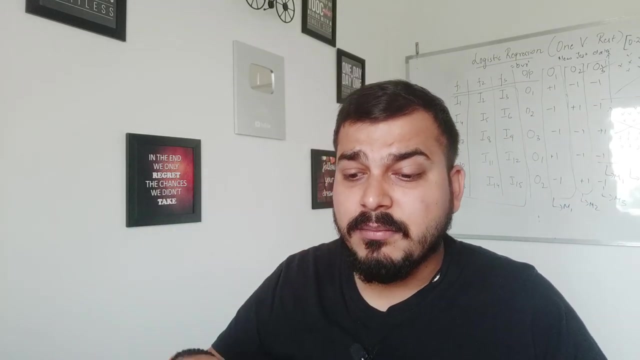 and high variance with respect to decision tree, and how you can actually convert the high variance into low variance. okay, and you can actually convert this high variance into low variance by using simple techniques of hyper parameter tuning, like decision tree pruning. okay, so this is also called as tree pruning. that basically means that you'll consider the decision tree. 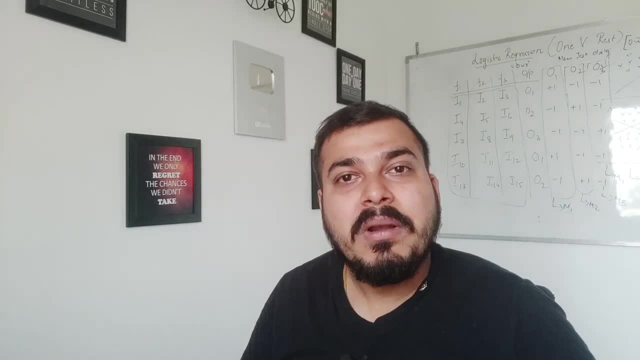 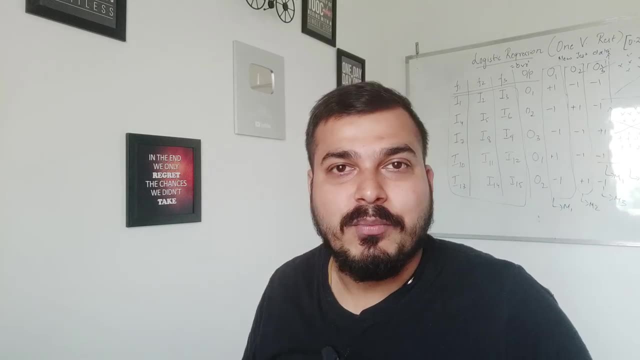 only till some depth, okay. you'll not go till the complete depth, till the leaf node over there, okay. so this is the kind of hyper parameter tuning and they'll also ask you that how you can perform that tree pruning steps and techniques. you should be able to explain that also. so it is pretty. 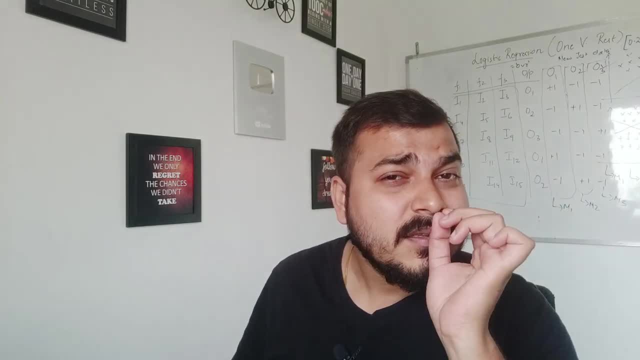 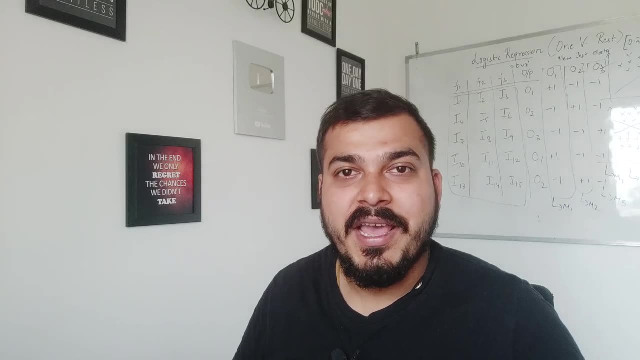 much important that you explain them now. this is also a very important question. they'll ask you the which are libraries which you you will be using in order to construct the decision tree, because constructing the decision tree will actually give you some of the visualization stuff you know you'll. 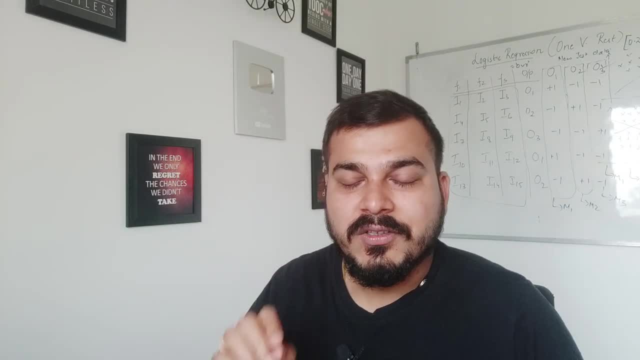 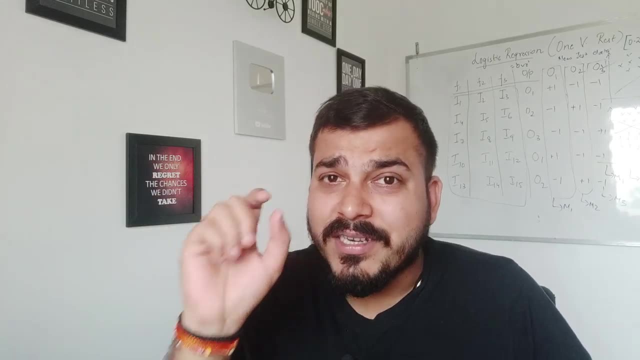 be able to understand how the decision tree looks like. okay, so here some of the libraries that they will definitely ask you, that which all libraries you actually use in order to construct a decision tree, and with respect to this also, i've created a video. have a look on to that particular video. 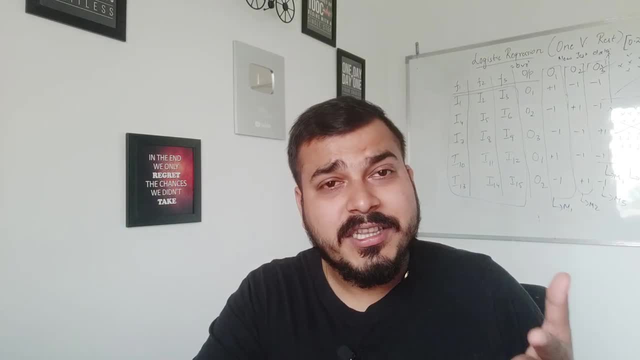 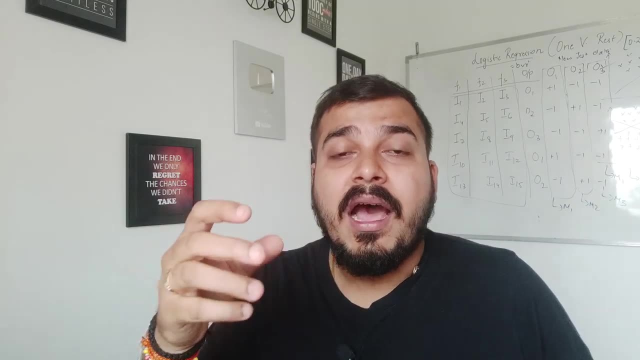 uh, you'll be able to understand all that, all, all, all the theoretical stuff that i've explained about decision tree, all the practical stuff also, and apart from that, you'll also be able to understand how the decision tree is actually splitted and how the decision is constructed. 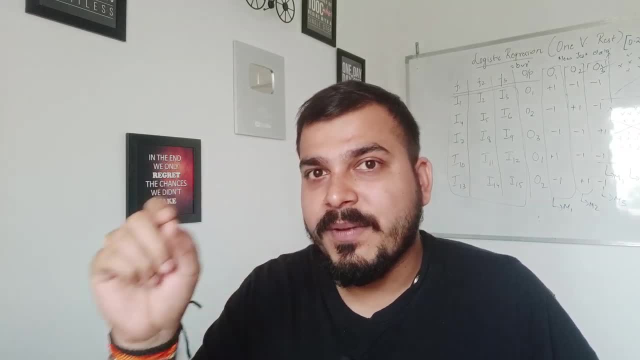 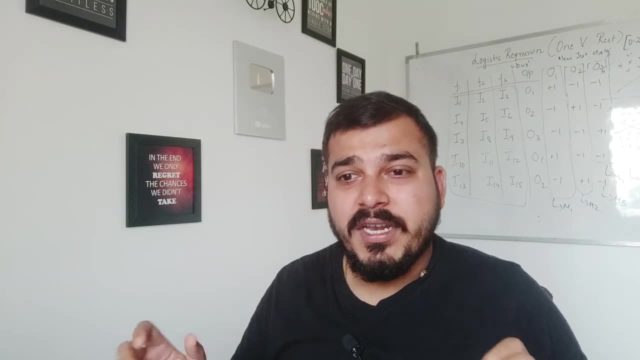 and it is also visualized, so make sure that you go and watch my complete machine learning with playlist there. i've explained everything about decision trees. so, yes, this was a short video on interview questions on decision trees and this was most probably asked to me by various 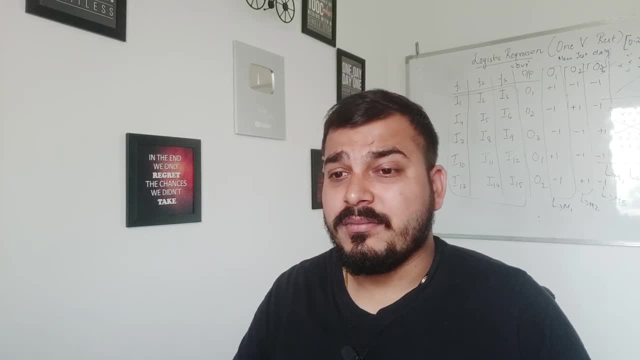 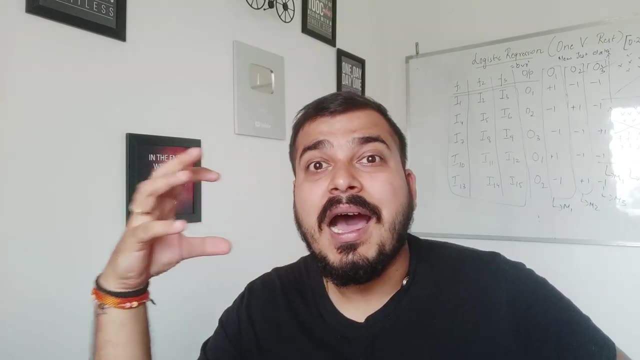 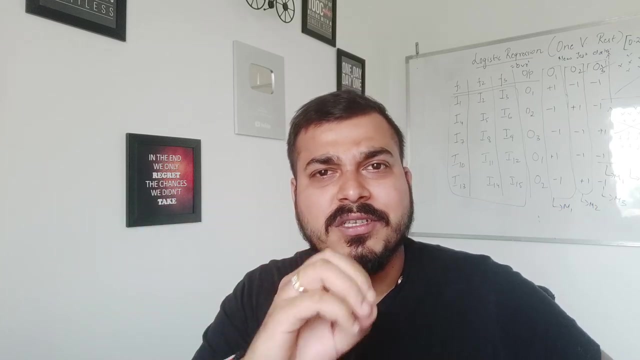 recruiters. so i have actually listed down, and this will cover everything, the outliers, okay, huh. one more question was pretty much important: how the decision tree classifier works and how the decision tree regressor works. okay, because many people- again i'm telling you, many students, many professional people. they just focus on decision tree classifier. 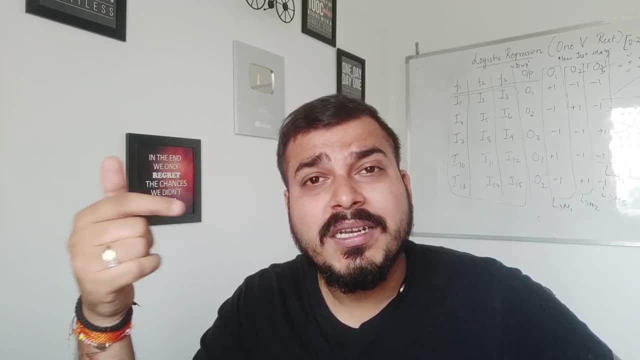 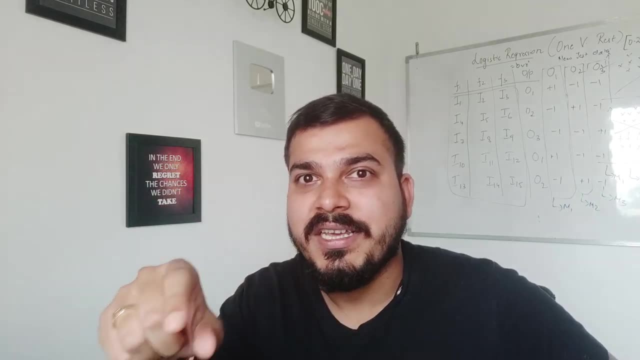 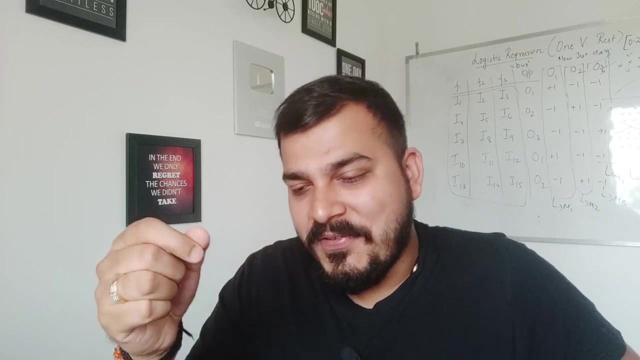 they don't know how decision tree regressor works. so you also need to understand the theoretical concepts behind decision tree regressor. in decision tree regressor, you will not have entropy, information gain and all okay. there you have something called as mean squared error, okay. so just try to understand in this particular way and if you try to explain them that in